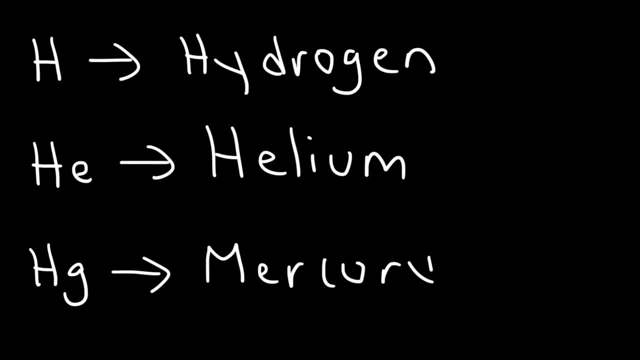 HG stands for mercury. Mercury is a special metal because most metals are solid at room temperature, but mercury is a liquid. So that's pretty interesting. Now let's go over the chemical symbols that start with a C. So we have C, CL, CA, CR, CO, CU, and then CD, CS and CE. 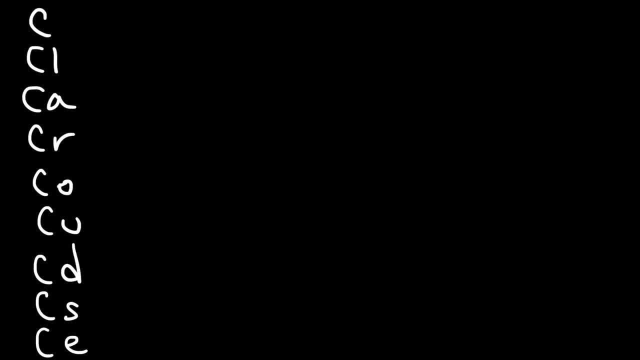 There's a lot of C's. There's a lot of C's that you need to know, And so it's very easy to confuse one with the other. So the first one C. this is carbon. Carbon is found in basically all living things on Earth that we know of. 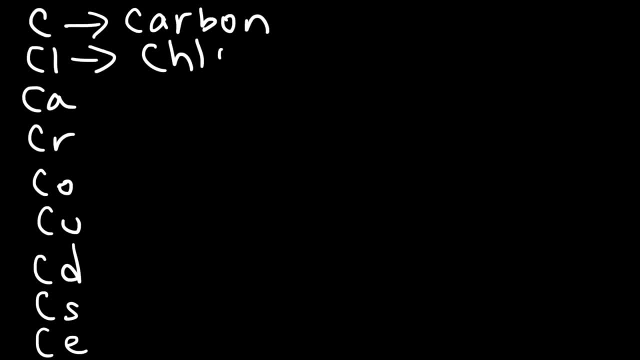 Next up we have chlorine. This is the stuff that people clean their pools with. CA is calcium. You'll need this to make strong bones. CR is chromium, CO is cobalt. Don't have much to say about that. one. CU is copper. 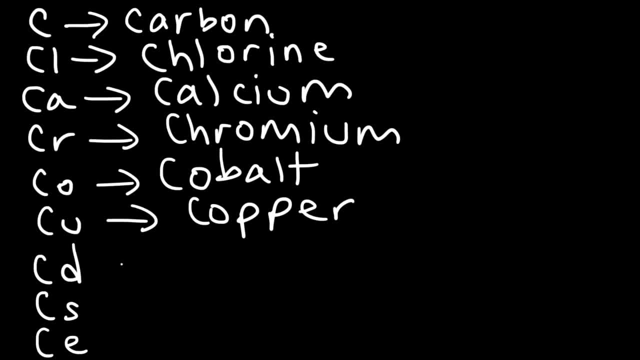 Typically, most electrical wires are made with copper. CD is cadmium, CS, that's called cesium, C-A-E-S-I-U-M, And CE is cerium. Now I recommend that you write the symbols and the names down for the sake of practice. 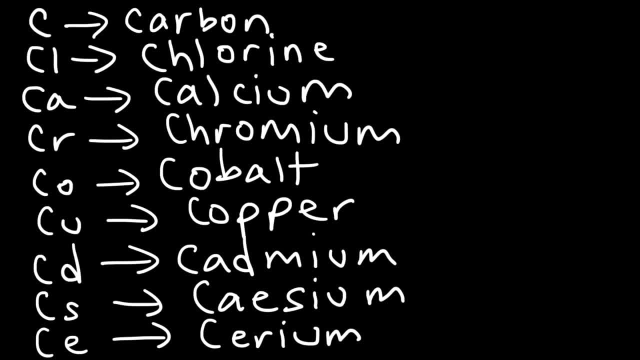 because later in this video I'm going to quiz you. I'm going to give you the chemical symbol and ask you to write the names, And I'm going to do it in a reverse order. I may even have a matching quiz just to help you to memorize the elements of the table. 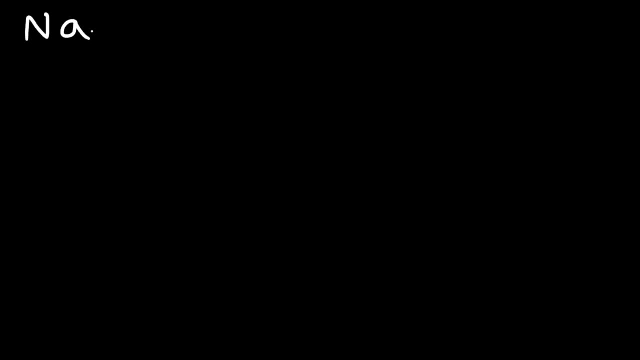 So now let's move on to the chemical symbols that start with an N. So we have NA, N, NE, NI and NB. So NA. what do you think NA stands for? Here's a hint: It doesn't contain an N. 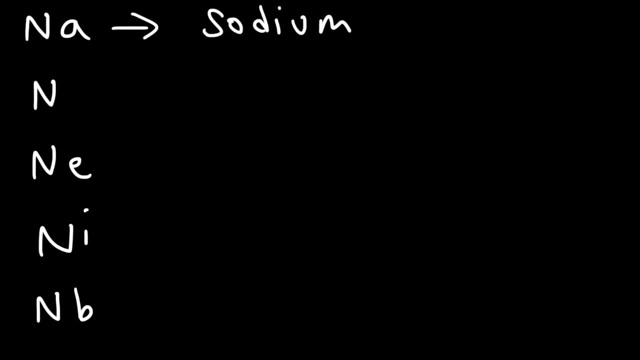 NA is sodium. If you put sodium metal in water it will explode. It's an alkali metal. It's very reactive, very dangerous. But sodium is also found in table salt, But it's an alkaline metal. It's in a different form. 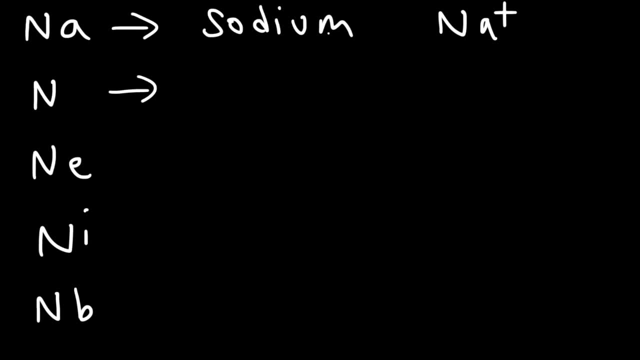 It's in the form of an ion as opposed to a metal. So in table salt it's completely safe, But as a metal very dangerous. N stands for nitrogen. Nitrogen is prevalent in the air. In fact, approximately about 78% to 79% of the atmosphere consists of nitrogen gas. 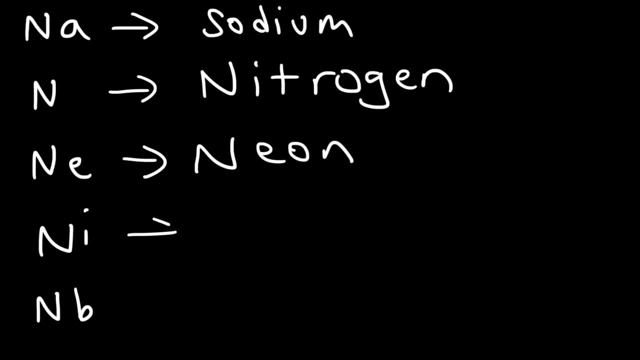 NE is neon. Think of neon lights. NE is oxygen, NI is nickel. Think of a five-cent nickel NB niobium. Let's hope you don't get that one on the test Now. I remember when I was in high school and I was taking AP chemistry. 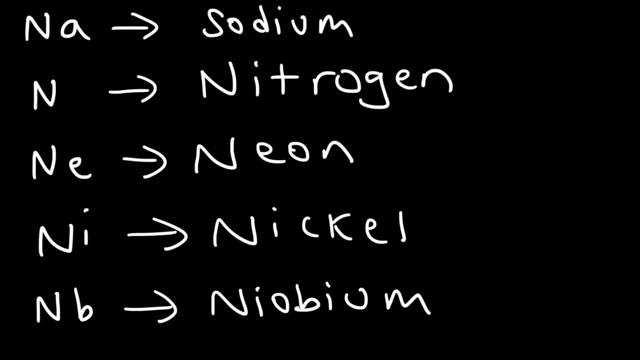 The next day we were given a pop quiz And we had to know 60 elements of the periodic table, And what really helped me was creating a mental image, a picture in my mind that relate an element with something familiar, And, at the same time, just quizzing myself. 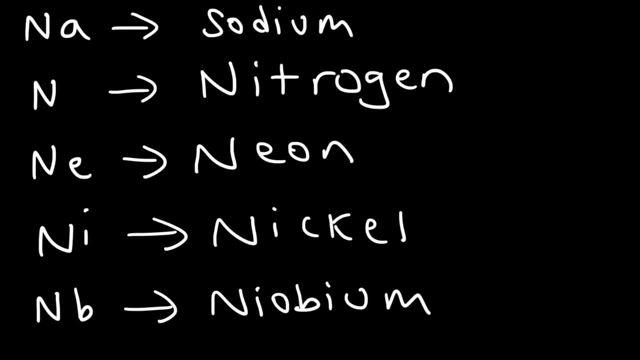 Just practicing by writing out the names of the elements and the symbols that go with it. I think that helped a lot too. Using the cards to match the name with the symbol And so doing that a few times helped me to pass that test or pop quiz. 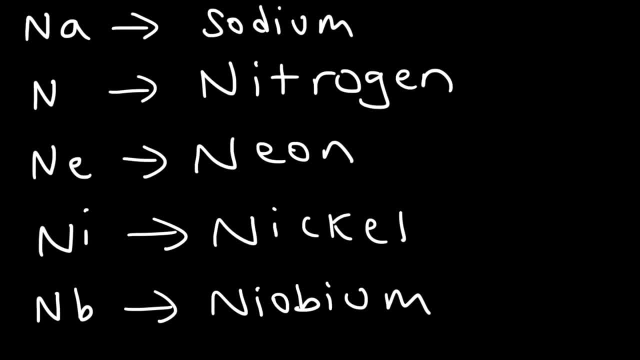 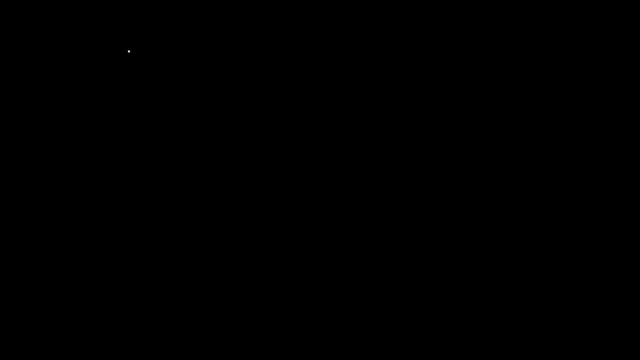 And that could help you too. So I definitely recommend That you quiz yourself if you wish to memorize the elements of the periodic table. Now let's go over the elements that start with an M. There's three of them that you need to know. 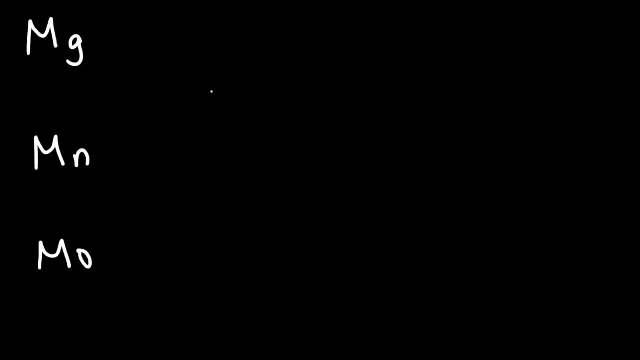 MG, MN and MO. MG stands for magnesium. If you take a magnesium ribbon and burn it in air, it produces this very bright white light And even ultraviolet, So you've got to be careful of that. It was one of the experiments that I had in my AP chemistry course. 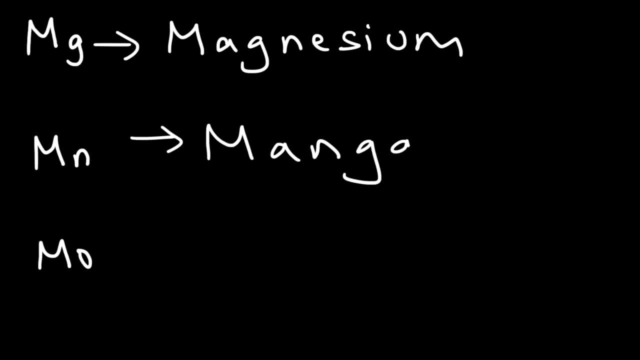 MN stands for manganese, And then MO is molybdenum. I really don't have much to say about those two. Now the next ones you need to know are the ones that start with a- B. There's B, BA, BE. 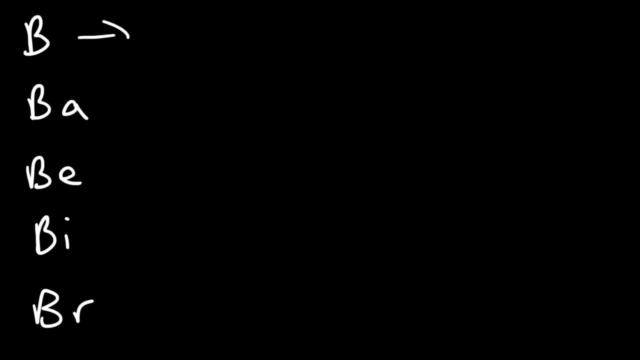 B, I and B? R. So BA stands for boron. I mean that's B, not BA. BA stands for barium, But B stands for boron, BE stands for beryllium. That's an R and then a Y. 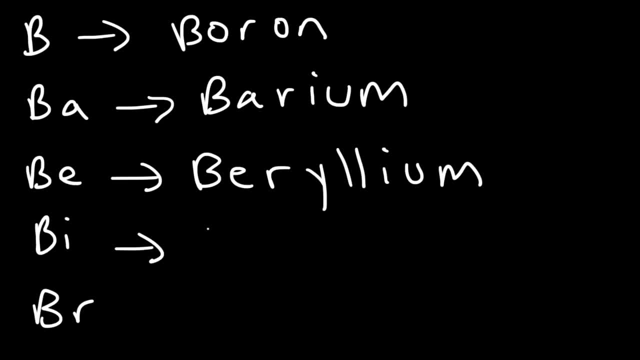 I kind of grouped those two letters together And then BI is called bismuth, BR is bromine. Bromine is a red liquid nonmetal at room temperature. It's also a halogen, And halogens are very reactive nonmetals. 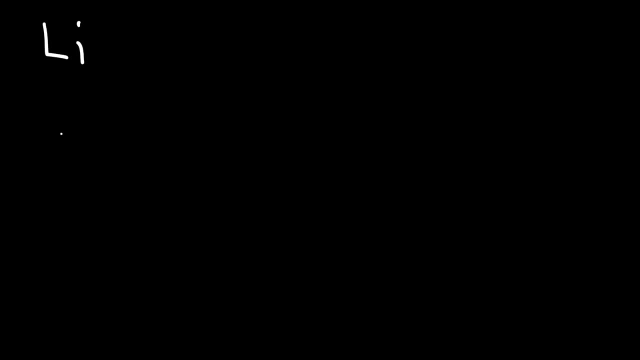 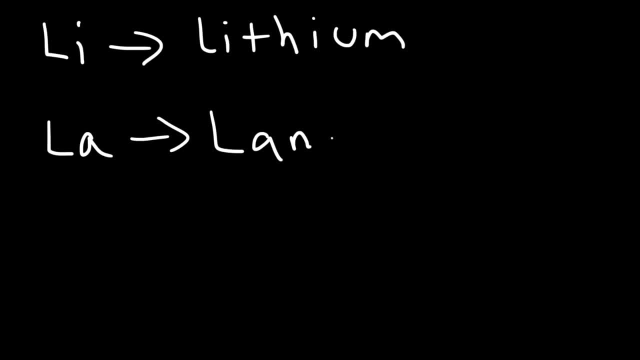 Laptops and cell phones. La is called lanthanum. Next we have O and OS. O, as you probably have guessed, is oxygen. OS is osmium. OS is osmium. Next we have the element F. Next we have the element F. 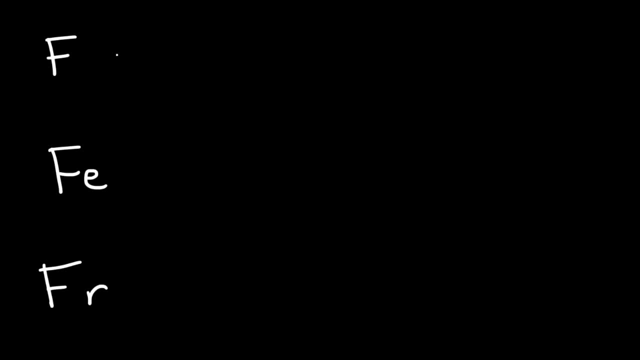 F is xylophone. Next, we have the element F and FR. So F stands for fluorine, The U comes before the O And you can find this element in toothpaste in the form of fluoride. FE is iron, even though it doesn't have an F in it. 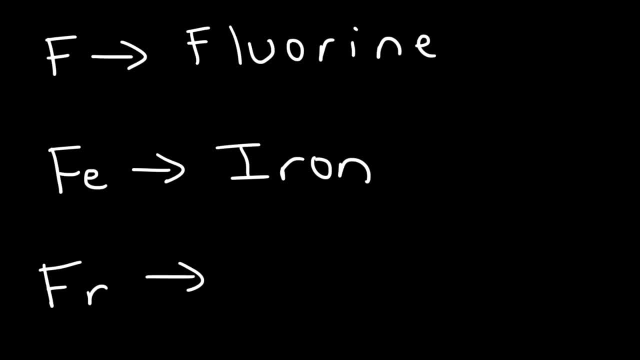 But iron is also known as ferrous. If you hear the word ferrous, it tells you that it basically has iron in it, And that's where the FE really comes from. So if you hear ferric or ferrous, you know you're dealing with the chemical symbol iron. 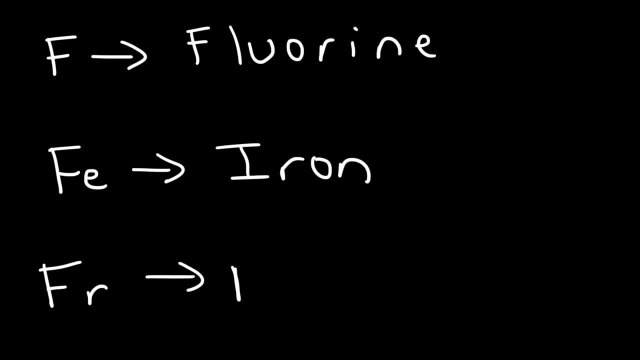 in different forms. FR is francium, It's another alkali metal. And next we have K and KR. K doesn't have a K in it. This is potassium, KR is krypton. Think about where Superman came from. Now let's move on to the chemical symbols that start with an A. So we have AL AS AR. 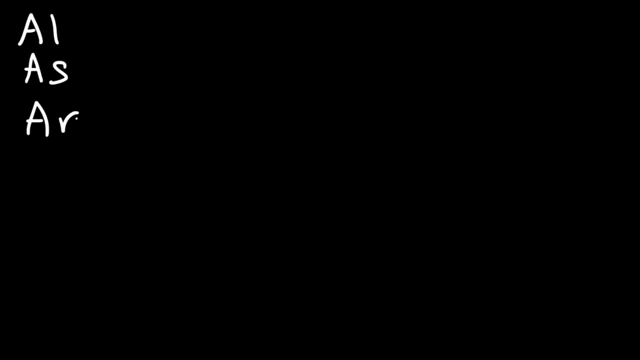 If you notice, the first letter of the chemical symbol is capitalized And the second one is in lowercase, So we have AGAU, AT and AC. Think of aluminum foil, which is probably in your kitchen- AS stands for arsenic. 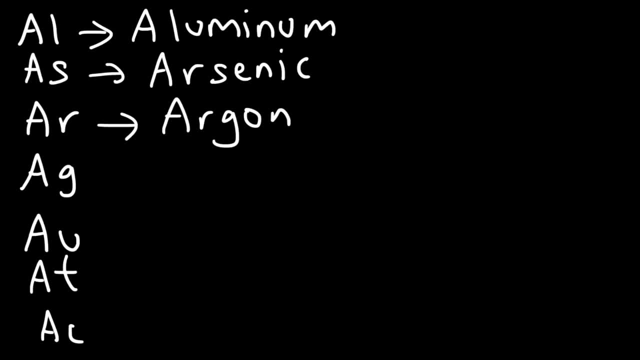 AR is argon. It's a noble gas that can be found in the atmosphere in low quantities. What do you think AG is? AG is a noble metal, but it doesn't have an F in it. Or can it be found in the atmosphere in low quantities? 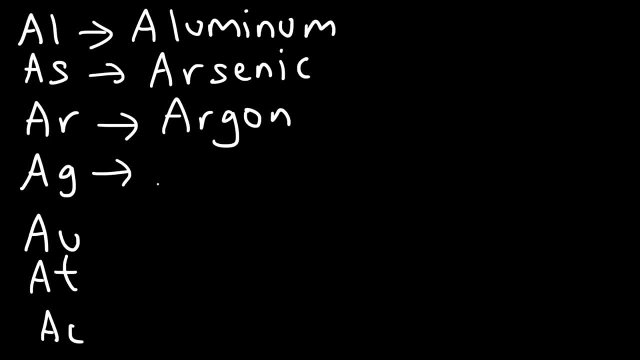 if you hear the word ferric or ferric. It's a noble metal, but it doesn't have an F in it, It's an Al. start with an a. AG is silver, au is something similar. doesn't start with an a either. au is gold. so these two are very common test problems. so make sure. 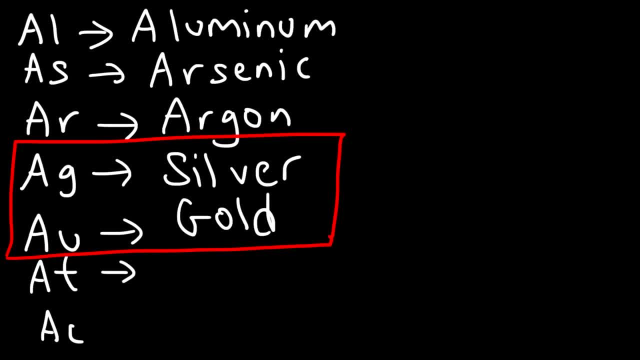 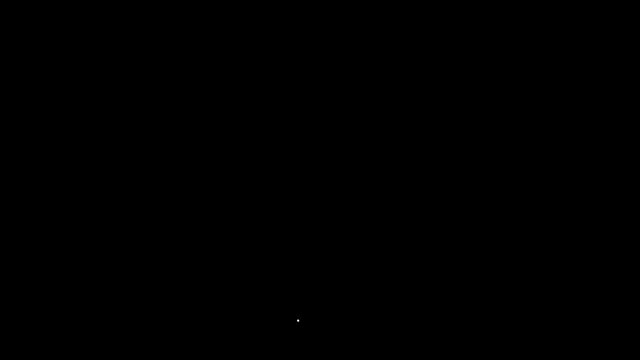 you know those two: AT is called astatine and AC is actinium. so that's it for the symbols that start with an A. now let's move on to those that start with an S. so there's SI. S has C, SR, SN, SB and SE. the first one, SI, is silicon. silicon is a metalloid. it's. 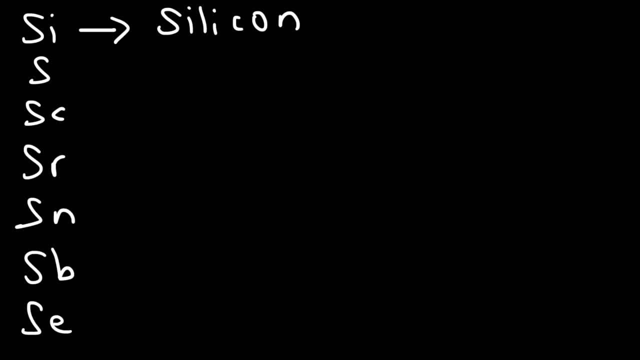 between a metal and a nonmetal. metals can conduct electricity, nonmetals do not, but metalloids like silicon and even germanium. they can conduct a small amount of electricity. in fact, silicon. it's found in many solar cells. a solar cell is a device that takes sunlight and 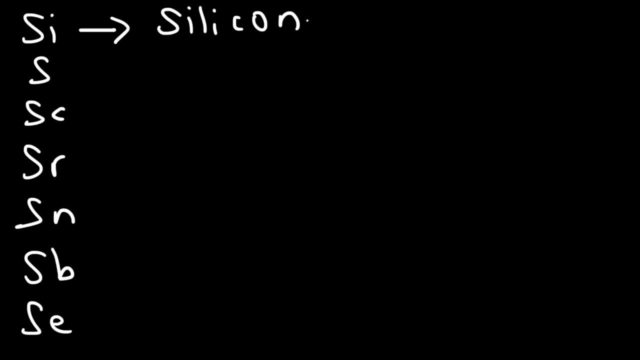 converts it into electricity, and you can find silicon in sand and glass. it's very abundant in the earth s stands for sulfur now. sulfur is basically a yellow solid, but when it melts it turns into this red liquid. c is called scandium and then sr is strontium. it's an alkali earth metal, SN. 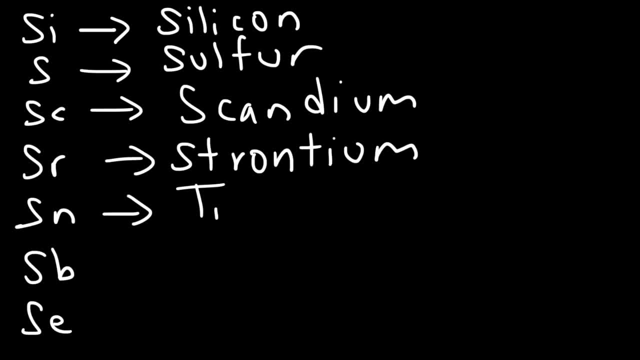 doesn't start with an s. this is tin metal, but i think it's latin name is like Stannis. if you see Stanek, it typically refers to tin metal. Sb is antimony and Se is selenium. Selenium is also another metalloid that is found in. 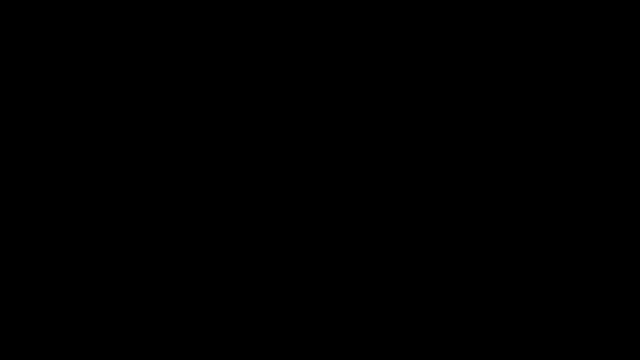 some solar cells. Next, let's go over the elements with symbols that start with a P. So we have Pb, and then there's P, Pd, Pt, Po, Pu and Pm. So Pb is very common. It's known as the lead. P actually starts with a P. This is phosphorus. Pd is 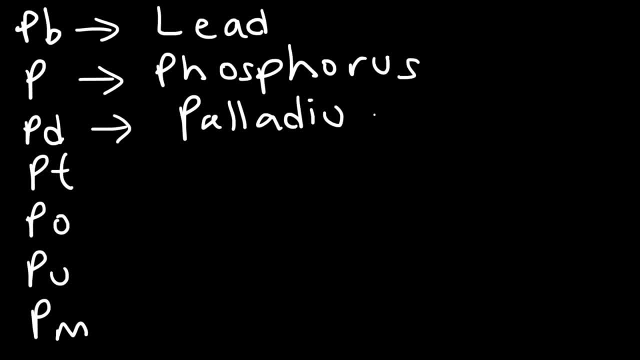 palladium, and PT is platinum. PO- this is called polonium and PU is plutonium, PM. you may not get this one on the test, or you may get it, but this one is called promethium. it's not too hard to forget this one. now let's move on to the elements that start. 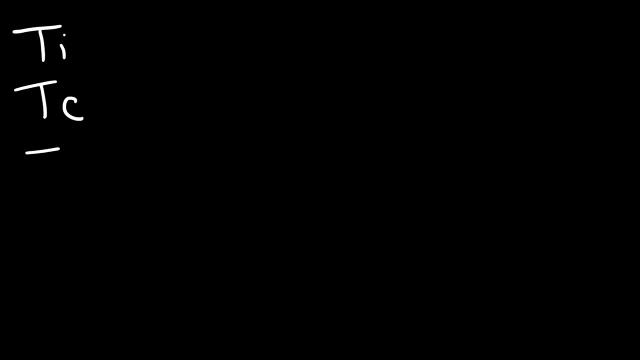 with T. so we have ti, TC, ta, TL, te and th. ti is titanium, it's another metal, TC is technetium, ta is tantalum, you, and TL is thalion. te, that's tell arium cl. easel's nutm goes with it. plahm, 네 chan, cars' nutma is an esos and ل. 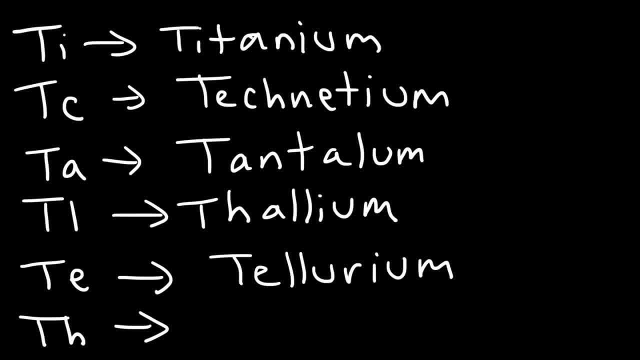 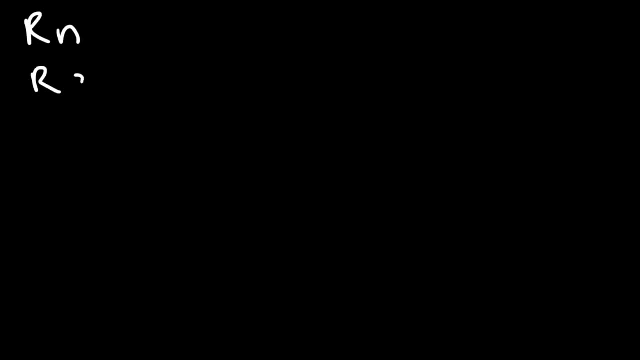 and T. c is thing that we have platy foam. TA is titanium and, plahm you, It's a chalcogen just below selenium on a periodic table. and TH is thorium. Now let's go over the ones that start with an R. So we have RN, RA, RB, RH, RU and RE. 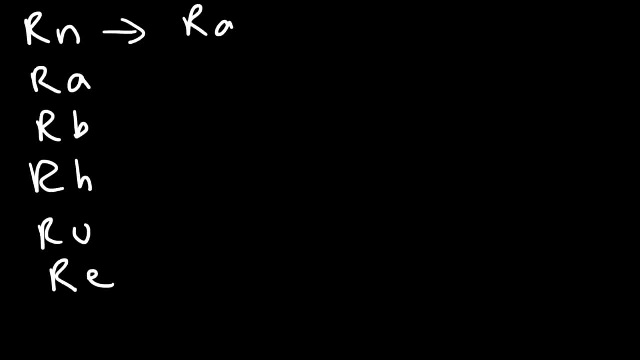 So RN is called radon. It's a noble gas that basically seeps from the ground and goes into the air For houses that are completely enclosed. let's say, if you live in a house and you don't open the window, the radon which seeps from the ground it can build up in your house. 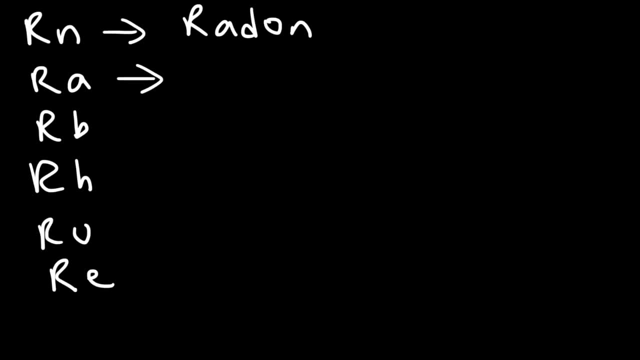 And so it's always good to open your window. RA is radium. RB is an alkali metal just under potassium. This is called rubidium. RH. this is rhodium. It's a transition metal. RU is next to rhodium. 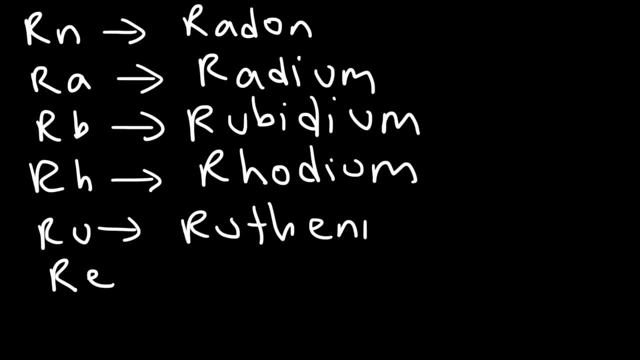 It's called ruthenium And RE is rhenium. So those are the elements that begin with R that you might be quizzed on. But most likely you'll see these three. They're more common. The other three you may be quizzed on it. it depends on your teacher. 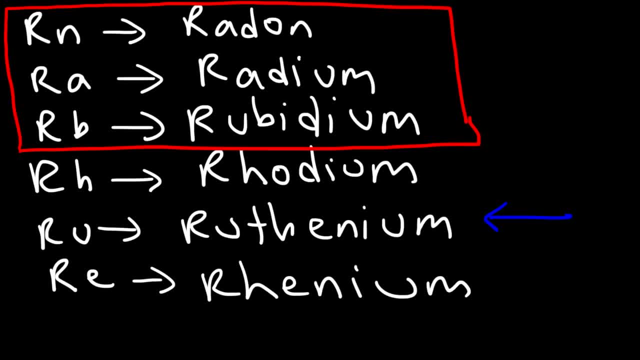 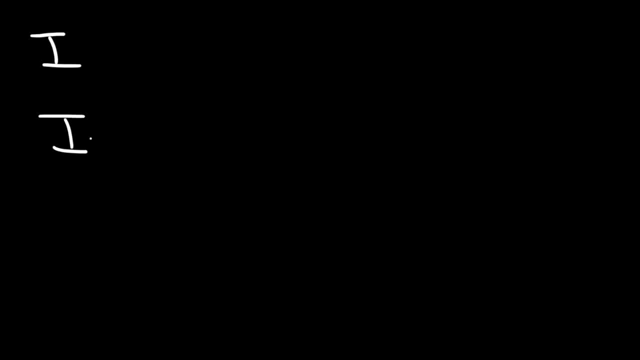 But they're less common, But you might see them occasionally. Now let's go over the ones that start with an I. There's I IN, And IR I stands for iodine. You can find this in iodized salt. IN is indium. 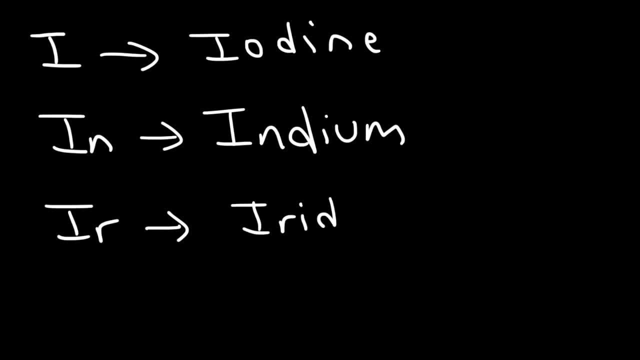 And IR is iridium. It's a transition metal with a high density. Now there's two elements that you need to know that start with a Z. The first one is zinc And the other one is zirconium. So you really shouldn't have a problem with these two, because you know this one starts. 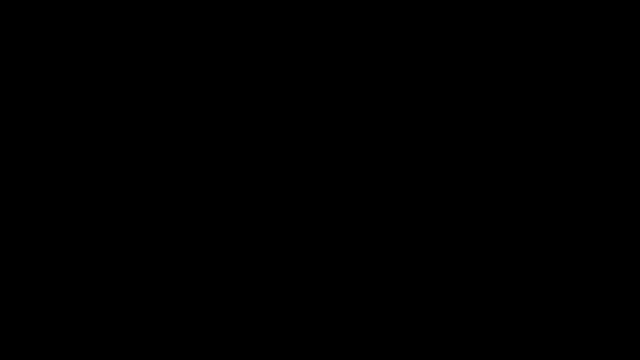 with an R and there's an R inside of it. Next we have GA and GE. GA is gallium, It's just under aluminum. GE is germanium- It's another metalloid That conducts electricity better than silicon, And the other one is zinc. 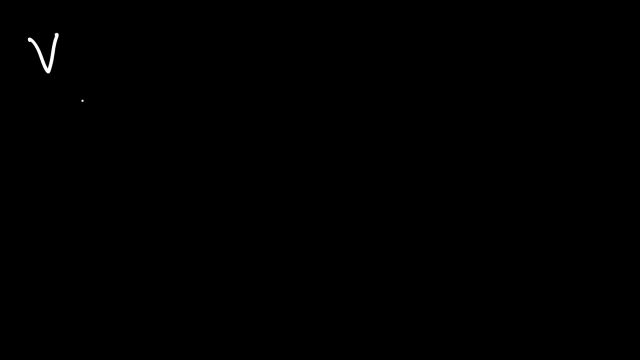 And the other one is zinc And the other one is zirconium And some other elements that we have that I'm just going to write them here so you can add this to your list. V stands for vanadium, XE is xenon. 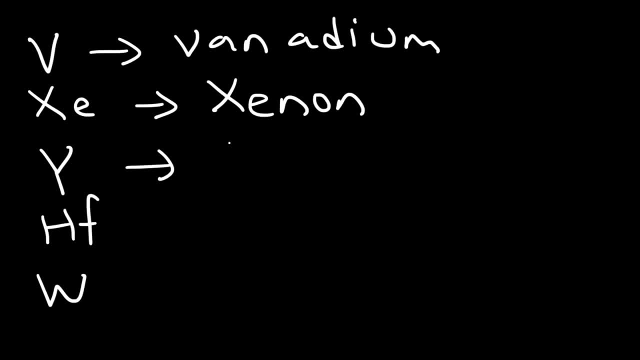 It's a noble gas, And Y is yttrium HF. This is called hafnium HF, And W is known as tungsten. Tungsten has a very, very high melting point. It's a metal that is very difficult to melt. 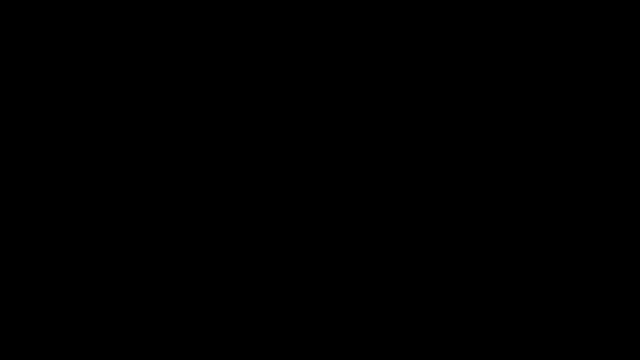 So let me give you a mixed review. I'm going to write a few chemical symbols And, while I'm writing these down, write the names of the elements that correspond to the chemical symbols. Feel free to pause the video If you wish to do so. 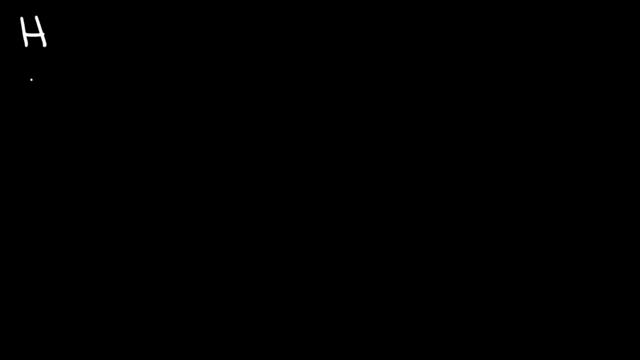 So what is the name of the element that corresponds to H, C, N, F, B-A, S, A-R, K, P-B, F-E, A-P-B, F-E, A-P-B, A-P-B, A-P-B? 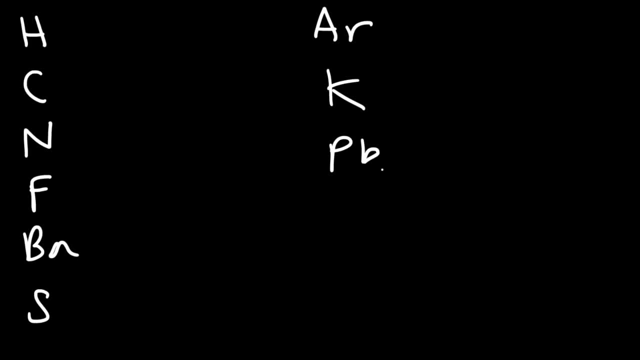 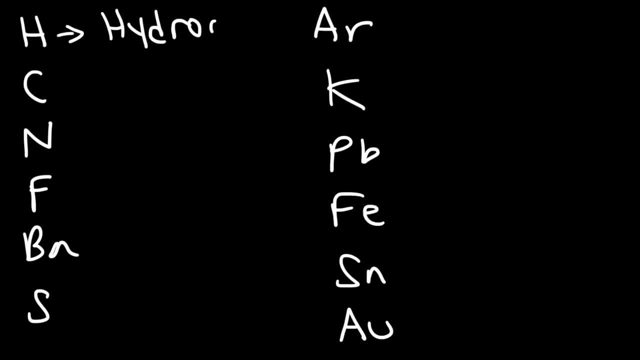 So H stands for Hydrogen. It's the first element in the periodic table. C is Carbon. You could find carbon in pencil lead, The mechanical pencils. If you take out that lead, Which the graphite form of carbon, and diamond is also pure carbon is another form of. 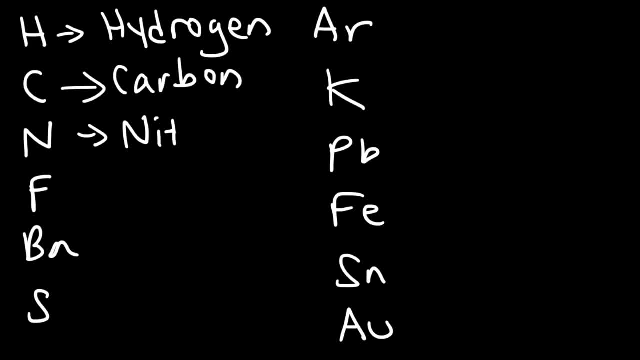 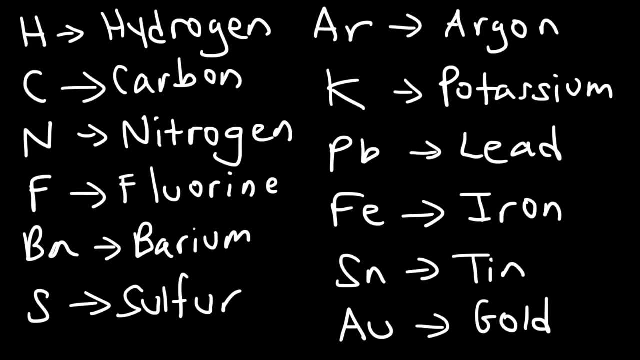 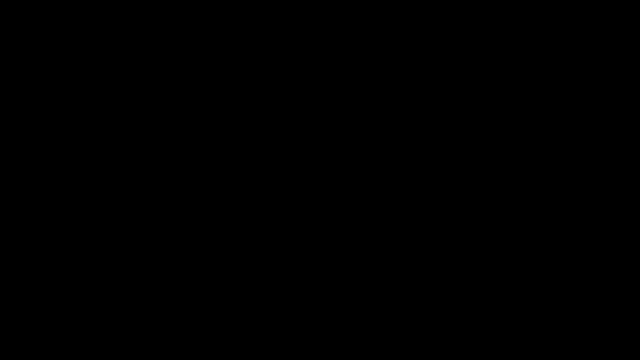 carbon and is nitrogen. F- this is flooring, BA is barium, s is sulfur, ar- this is called argon, k is potassium and PB is lead. Fe is iron, SN is 10 doesn't start with an S and au is gold. it doesn't start from a. now for the second quiz. i'm going to write the name of the elements and I 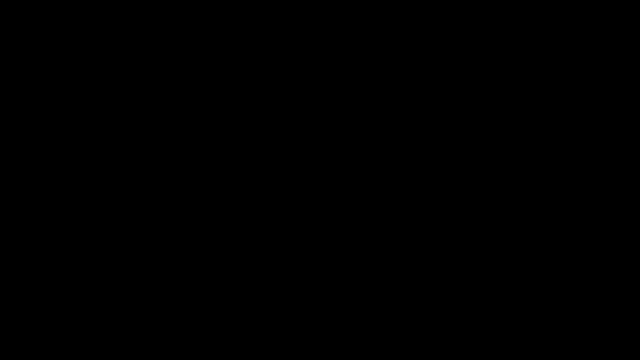 want you to write the chemical symbol. so it's basically the reverse order of the last problem set. so the first one is going to be magnesium and write the chemical symbol that corresponds to it. Next it's going to be silver and then sodium, and then bromine, After that calcium, cobalt and then copper. After that let's see. 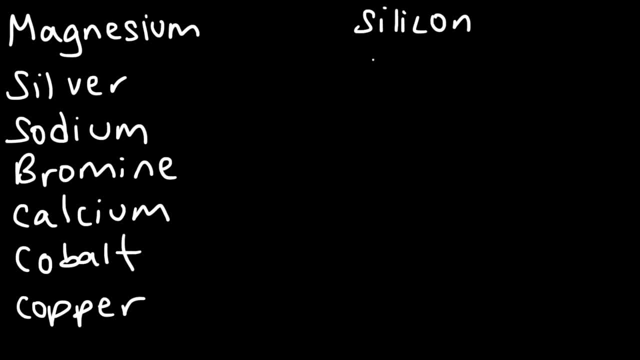 silicon, Let's go with iodine, zinc, platinum, radon, radium- Let's say magnesium, antimony and selenium. So go ahead, take a minute, pause the video and write the chemical symbols. that corresponds to the name of the elements that you see on. 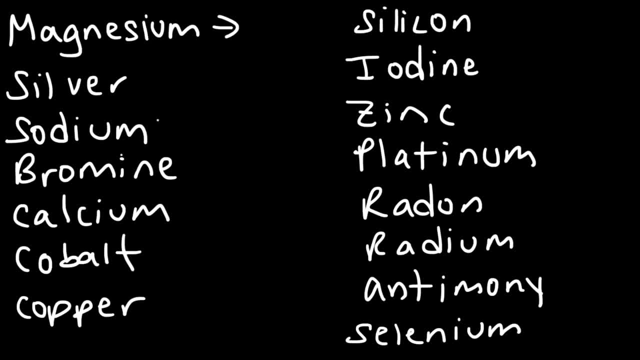 board. So magnesium is Mg. Silver- this is Mg. So magnesium is Mg. So magnesium is Mg. So sodium is Ag, Sodium is Na. Bromine- this is Br. Calcium is Ca, Cobalt is Co, Copper is Cu, Silicon is Si. Let me write that better. Iodine is simply I. 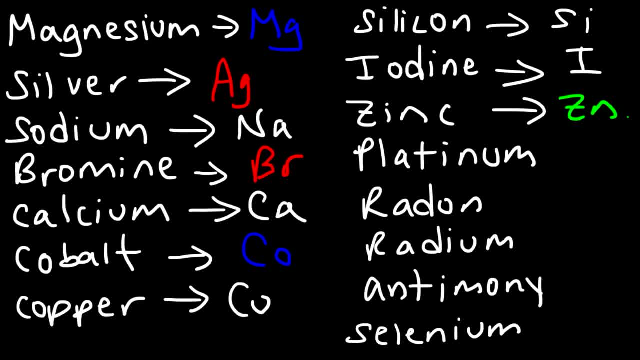 Zinc is Zn. Platinum, that's Pt, And then radon. this one is Rn. Radium, that's Ra. What do you think antimony is? Antimony doesn't start with an A, It's Sb, And selenium is 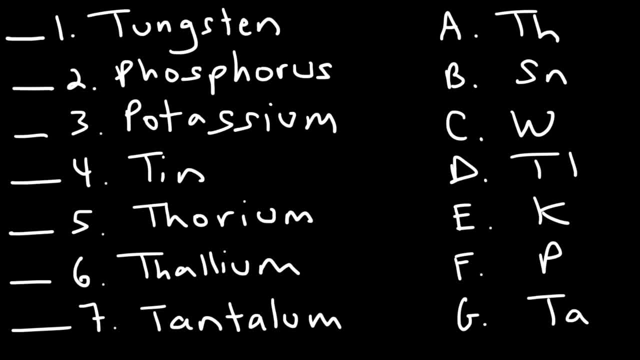 Se. Now here's a matching question. Here's a quiz that you can try to test your memory. So take a minute and work on these problems. So let's start with tungsten. Which one could be tungsten? Tungsten doesn't start. 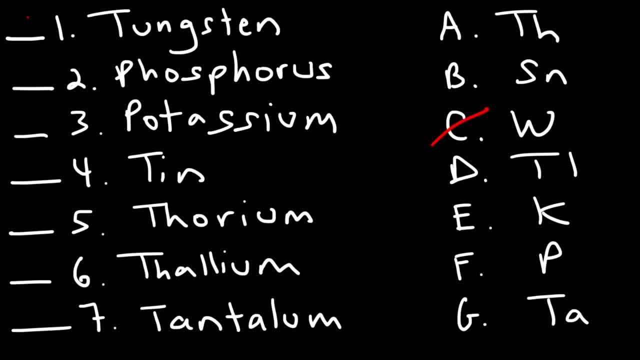 with a T. In fact it's a W. So number one is C: Phosphorus. Phosphorus starts with a P, But what about potassium? I was supposed to put an F here, not a P. Potassium doesn't. 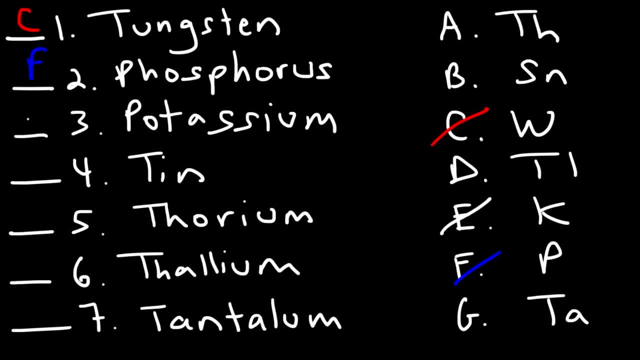 start with a P, Potassium is K, So that's the answer, choice E. And then tin doesn't start with a T, Tin is Sn. I was going to put Sn And then thorium, Thorium, that's not Tl. 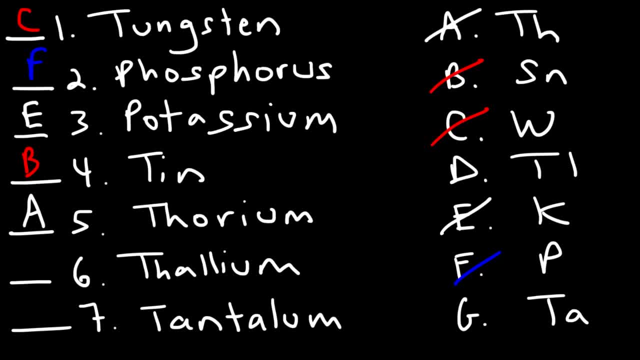 but that's T-H, so answer choice A. And thallium, that's T-L, so that's answer choice D. And the last one, of course, tantalum, that's T-A. So that's it for this video. 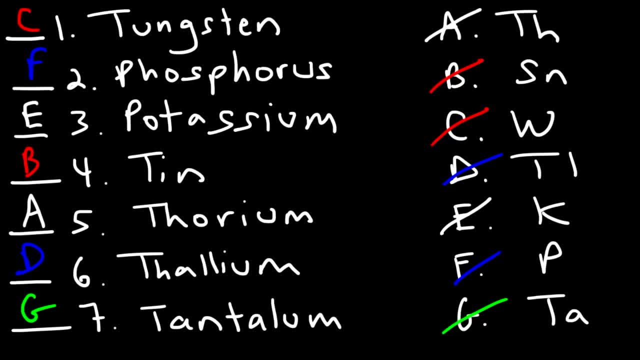 I highly recommend that you practice these types of problems And you can go to Google Images and type in periodic table elements, quiz or worksheet And just test your memory, because this will help you to pass the quiz that you're studying for And for those of you who wish to subscribe to this channel, that is, if you're thinking about doing that. 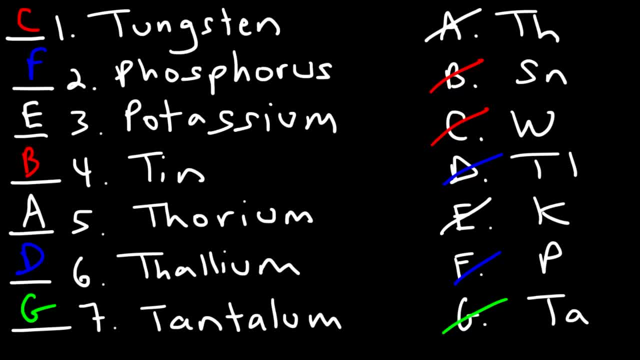 I highly recommend that you click the notification bell, Because currently I have around 300,000 subscribers And when I post a video, not everyone sees it. Maybe only 1,000 people may see it in the first day or so, So if you want to, 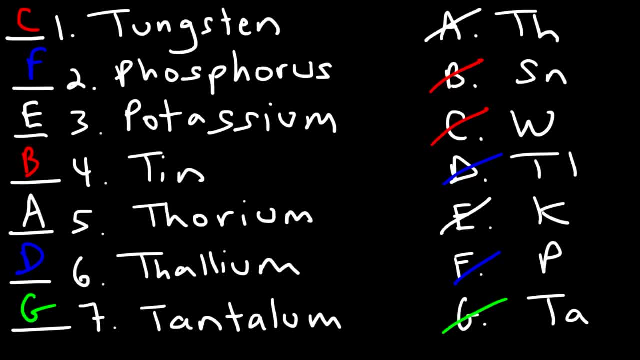 see any new videos that I upload on chemistry or other topics, feel free to hit that notification bell next to the subscribe button. In addition to that, for those of you who are studying chemistry, if this is your first time, check out my new chemistry video playlist. 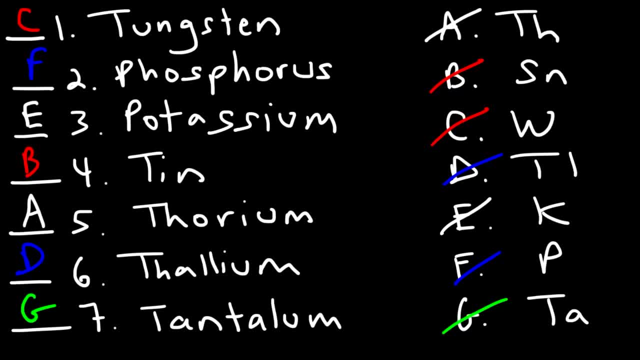 I'm going to post it in the description section of this video, But it's going to help you throughout your chemistry course, So feel free to take a look at that And, if you wish, to basically check out my channel. I do have other topics like 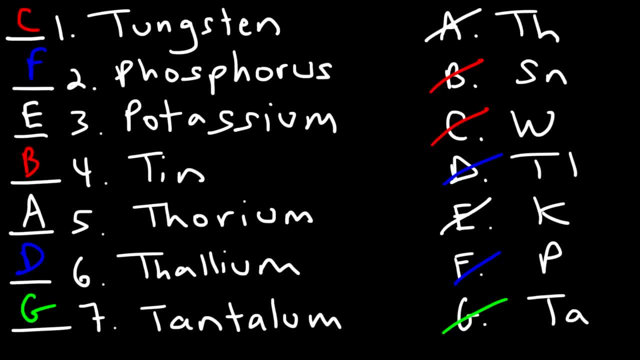 Physics, Algebra, Calculus, Trig, Precal. So if you're taking any of these math classes- or physics, that's another science class- feel free to check out the playlist that I have posted on my channel, Because that can help you as well. 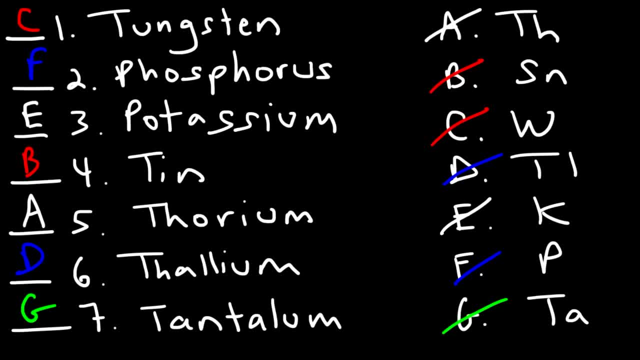 And thanks again for watching. So if you liked this video, feel free to comment, like, subscribe or share it with your friends.